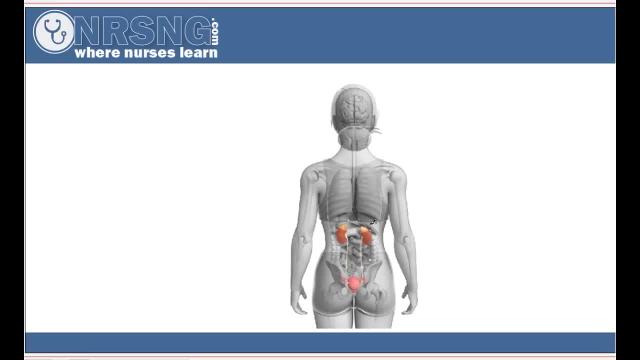 you can assess kidneys by percussing on the back of the patient just below the costal ridge there and you can actually feel, or the patient may. you can elicit pain of patient. if elicits percussing there elicits pain, the patient may be experiencing. 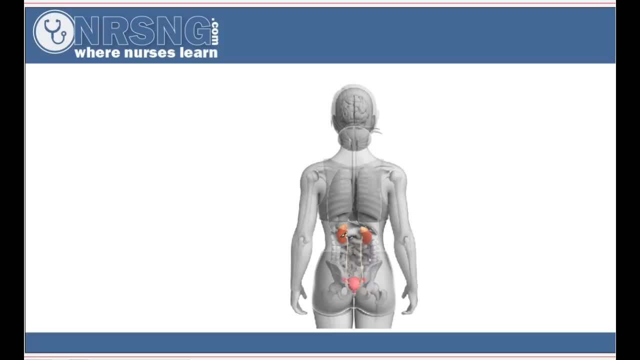 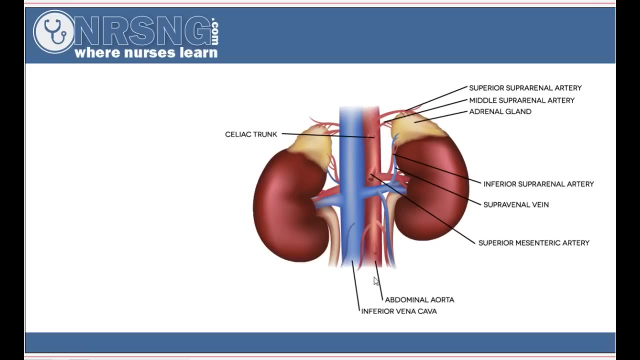 renal damage there. So that's how you can kind of check for the. that's where the kidneys are and that's how you can kind of check for them there. So really quickly let's just kind of talk about the external anatomy of the kidney. So blood is supplied to the kidneys from the abdominal. 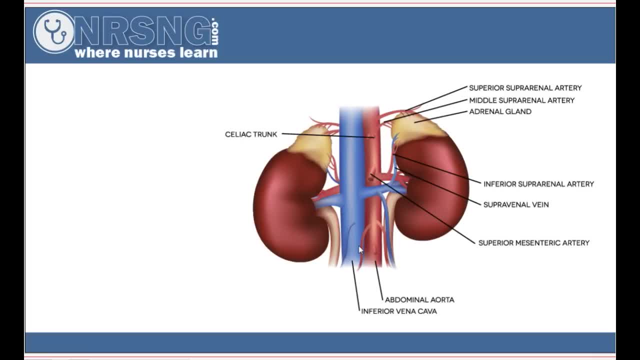 aorta and it's taken away from the kidneys via the inferior vena cava and the kidneys actually get about 22 percent of cardiac output. So they take up, they require or demand quite a bit of our cardiac output and you can see on top of each kidney you 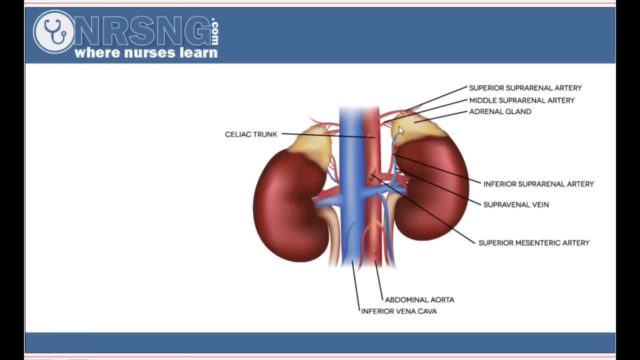 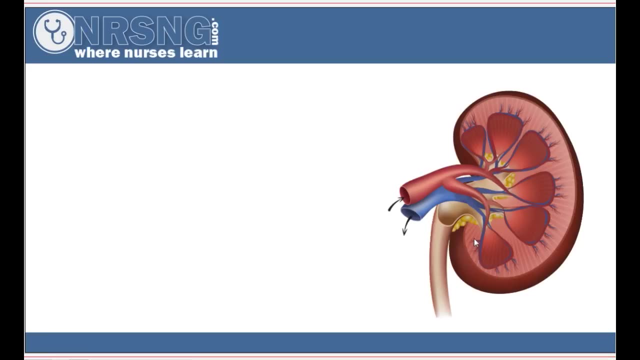 have your adrenal gland- and we've talked about that in different podcast episodes and things, but each kidney has a little adrenal gland on top of them and, again you can see, the right one is located just a tad bit lower than the left one. Okay, so then in inside each kidney, what we have here is 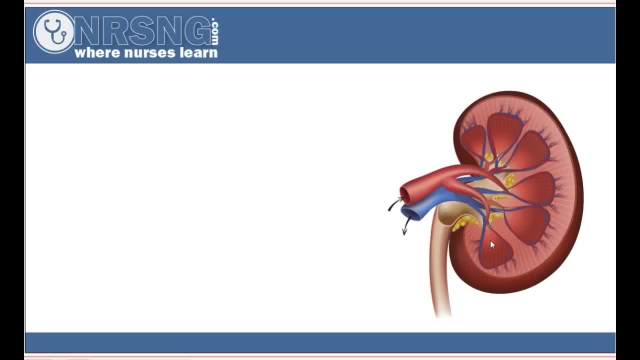 you can see these little darkened areas and you can see the adrenal glands and you can see the pancreas. These are called the pyramids, and within the pyramids you have this lower area here that's called the medulla, and then you have the cortex up here. Okay, so you can see. you have several of those. 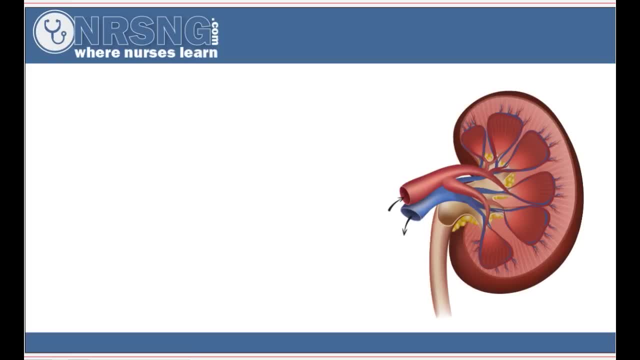 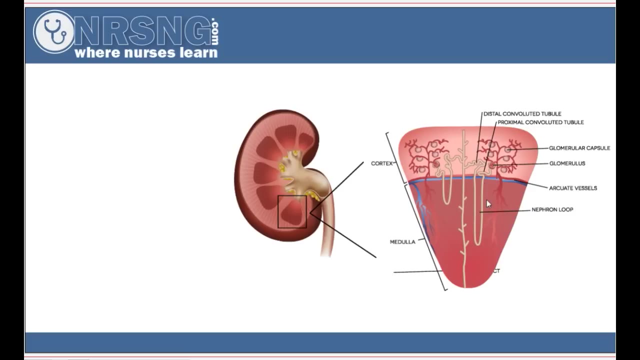 and then within these pyramids, we have, let's see here, within these pyramids, we have our nephrons. Okay so you can see here, this is the nephron kind of right here, and each kidney has about 1 million nephrons. Okay so, and 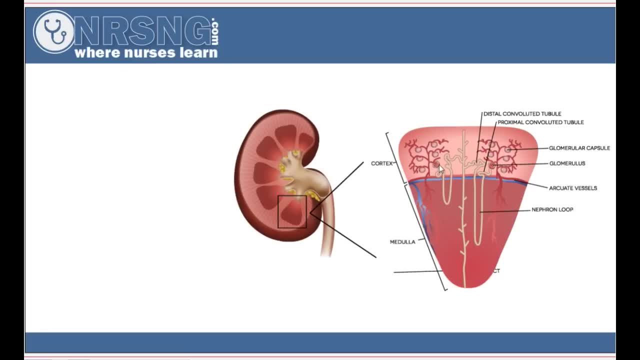 then up on the cortex, we have these little balls here. These are called the glomerulus. Okay, you can see the glomerulus. So what happens is blood is supplied, it eventually gets to here and in the glomerulus some of that blood is filtered and what is excreted then comes down here through the 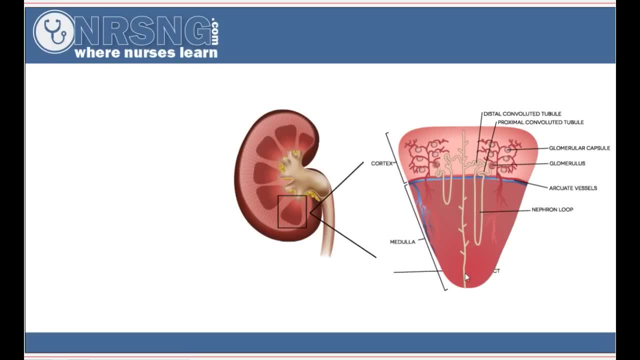 the loop. you know it's the loop of Henle, and then it is taken out via the collecting duct and then taken to the ureter and is excreted via the urine. Okay, so that's kind of how that all works there within the kidney. 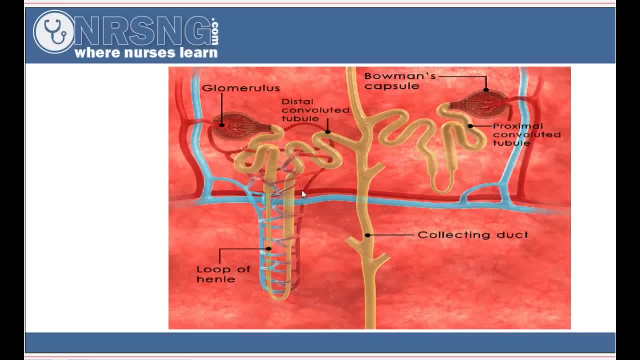 Alright, so a little bit closer. look. here you can see your glomerulus. here your artery is supplying the blood. here it's filtered and then it comes down. you have more blood coming in Here and some of it passes into the collecting ducts. the loop of Henle taken into the collecting duct. 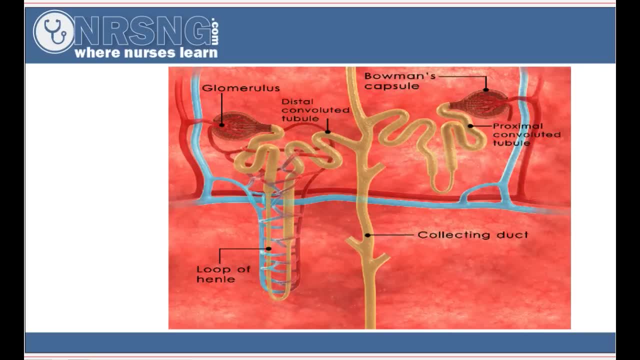 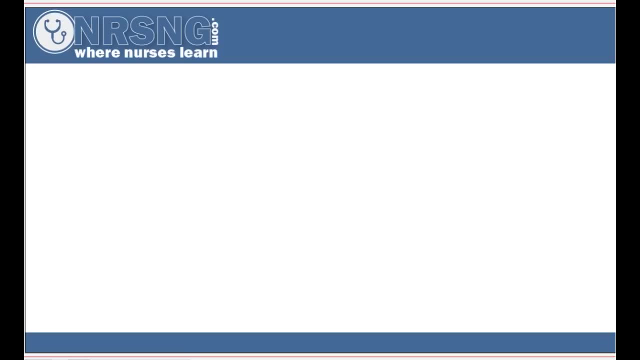 Okay, so that's kind of how it works in a very close range. looking at it much closer, Okay, so let's go back to this picture here. So what happens here is the liver, so blood urea nitrogen is a measure of how much. 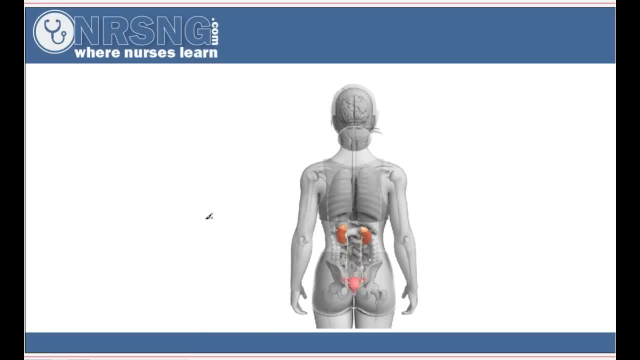 nitrogen is contained within the blood. Okay, so what nitrogen is? so what happens is your liver? we'll just draw a little liver here. There's a little liver, so what happens is nitrogen is actually a byproduct of protein metabolism. So when it's it's, it's created, or the urea is formed by the liver and its carried by the blood to the kidneys for excretion. 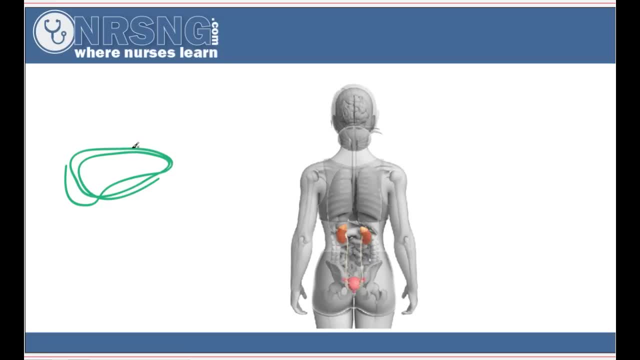 As protein is metabolized, it is then broken down into urea, And then urea travels from the liver and into the kidneys for excretion. So what can happen is, if you have decreased renal function, of course you are then going to see elevated BUN. 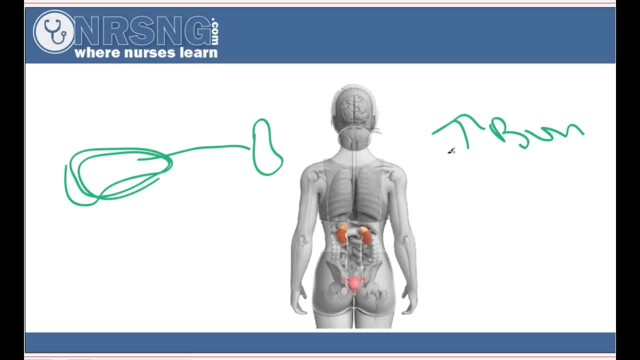 Okay. so if the kidneys are not able to appropriately filter this urea out and excrete it via the urine, you're going to see the BUN go up. Okay so, as blood passes from the liver, passes into the kidneys, it's going to pass through that whole little system that we showed there. 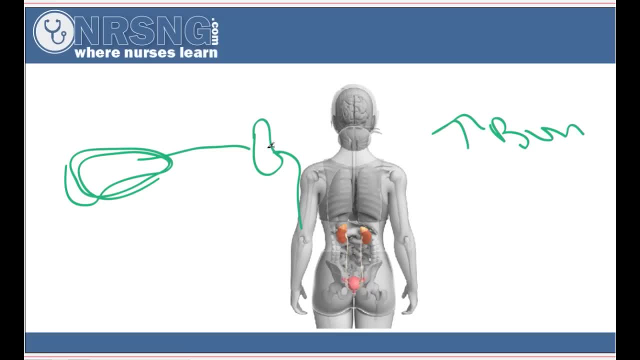 And then if it is unable to filter out that urea, you're going to see an elevated blood. Okay, so the reference value is going to be about 7 to 20. And values can decrease with pregnancy and then they can increase a bit with elderly patients. 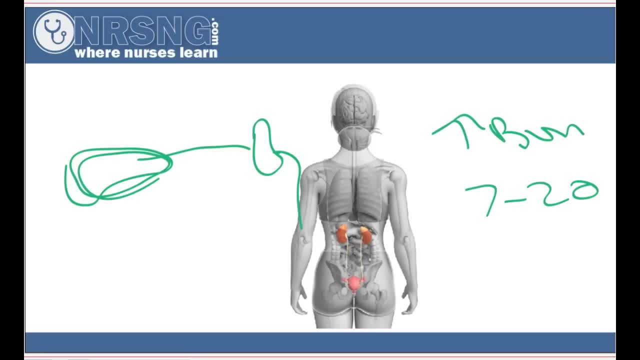 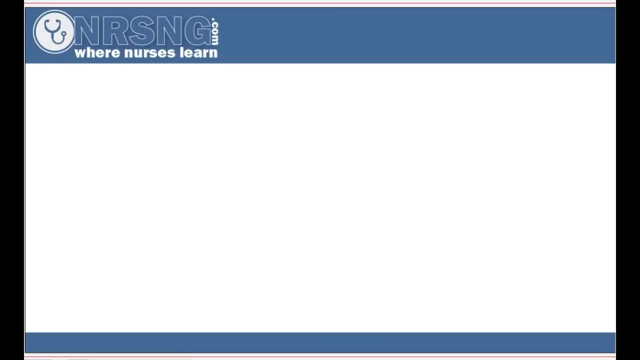 So let's talk about some of the different things that are going to lead to elevated or decreased levels, Okay so, Things that are going to increase your BUN, Okay. so if we're talking about increased BUN, what we're talking about is we're talking about the fact that the kidneys are not filtering that urea out. 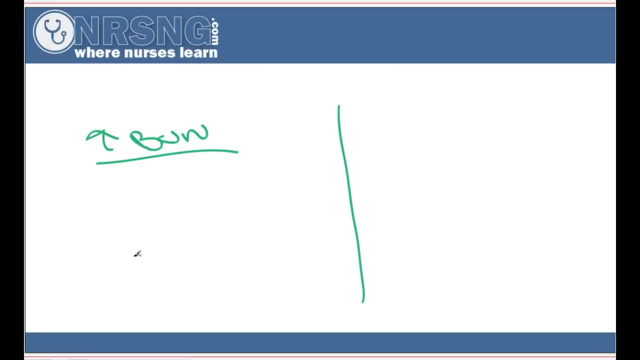 And so we're retaining that urea within our blood. Okay, so what are things that are going to increase the BUN, Or in other words, what are reasons that the kidneys may not be able to filter some of that urea out? 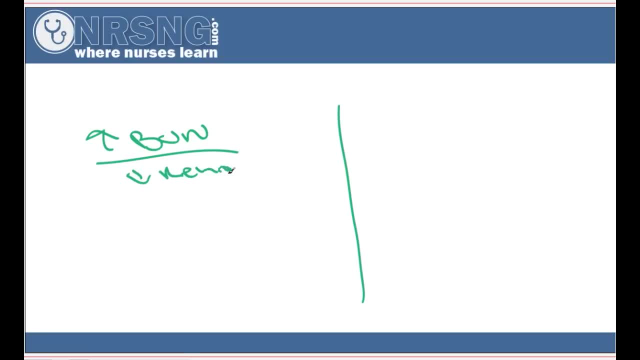 Okay. so of course, we're going to have decreased renal function. That's going to be one thing, CHF, Because we're going to have decreased blood supply to our kidneys, Dehydration, Shock, Hemorrhage, Let's see, let's write it like this: 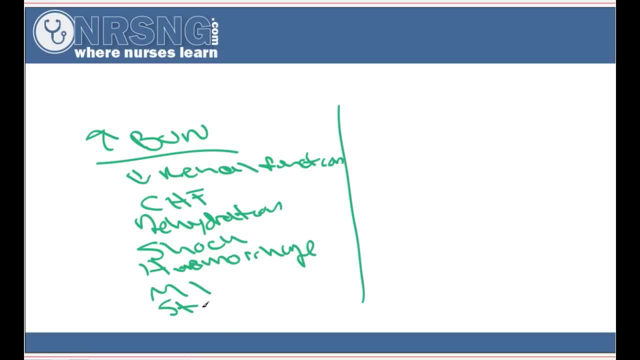 Hemorrhage, MI Stress And excessive protein intake. So, as we look at these reasons, these are all things that are going to. So this is just acute decreased renal function, So the kidneys themselves are not functioning as they should. These things here are going to be decreased blood supply to the kidneys. 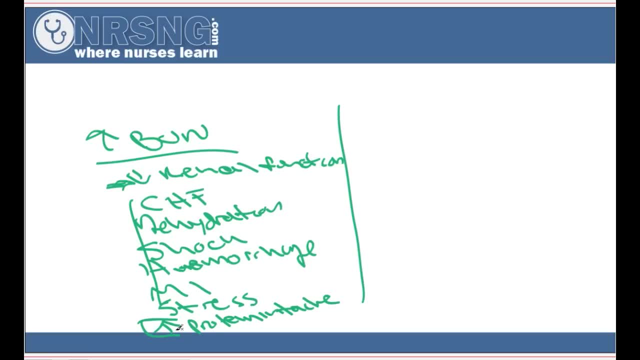 And then this, of course, is going to be increased protein intake. If we increase our protein intake, of course we're going to have more protein breakdown And the liver is going to deliver more urea and nitrogen to the kidneys themselves. 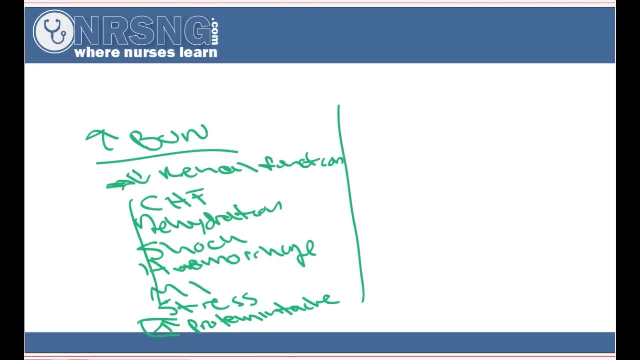 Okay, So let's talk about reasons that we're going to see decreased BUN- Okay, So, let's do decreased BUN- Okay so reasons that would lead to the kidneys excreting less urea- Okay, Okay. So some of the reasons for that would be: 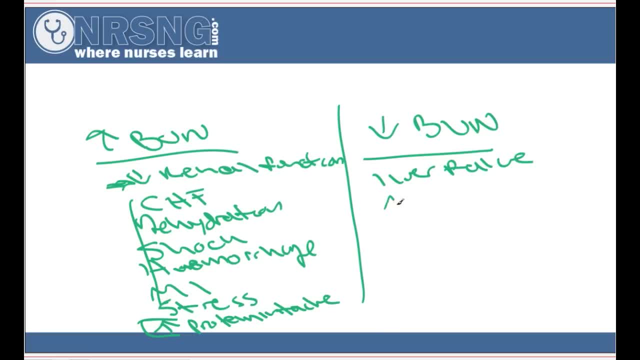 Liver failure, Malnutrition, Overhydration And SIADH. Okay, So we're talking about, And then like malabsorption issues- Okay, so again you've got to kind of think of the exact opposite reasons that we would have increased. 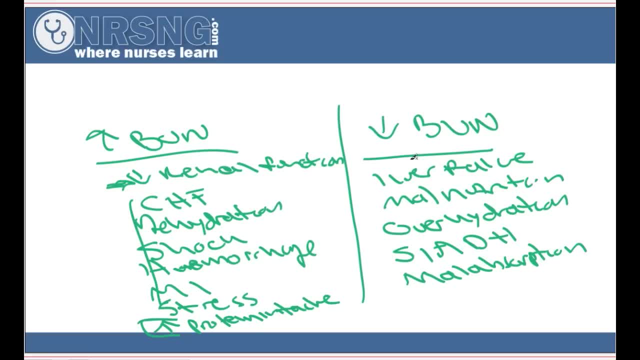 Because For decreased BUN, if our liver isn't working appropriately, it's not going to be breaking down and metabolizing protein, So it's not going to be delivering urea to the kidneys for them to excrete, And malnutrition if the patient's not getting enough protein. 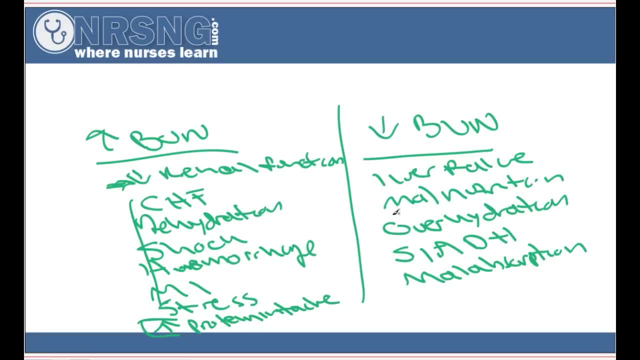 then again there's not going to be that urea delivered to the kidneys And then SIADH. So what can happen here is when a person has SIADH, the antidiuretic hormone response, It's responsible for stimulating the kidney conservation of water. 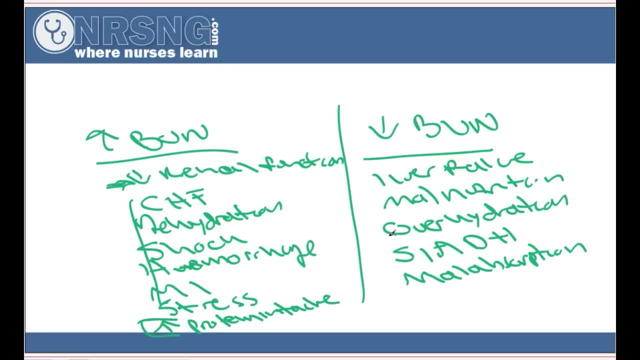 Causes excess water to be retained. So rather than excreting that water in the urine, it's retaining that water and it can cause the BUN to actually then decrease. Okay, So you're retaining all that water. blood's more dilute. 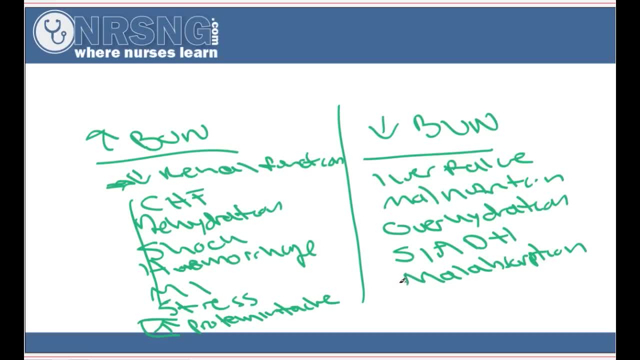 and you're going to have a decreased BUN. Okay, And then malabsorption, of course, even if the patient, If the patient's getting appropriate protein intake, if they're not absorbing that, then again the liver's not going to be breaking that down. 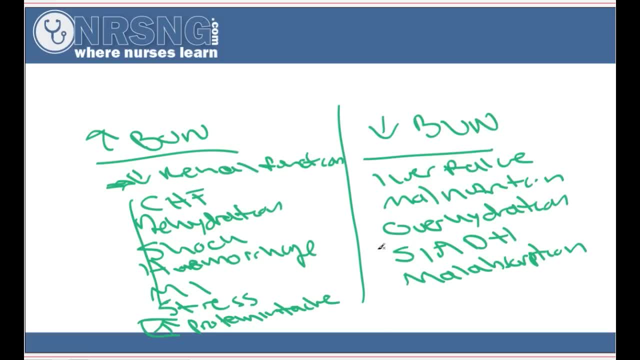 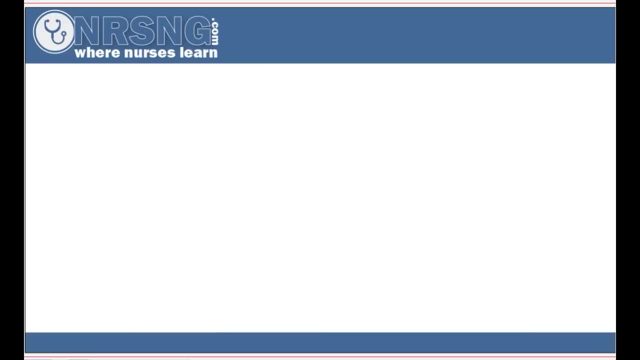 and it's not going to be delivering it to the kidneys. Okay, So those are just some of the things that can cause increased and decreased BUN- Again the thing we want to just think about really, just as a quick overview.